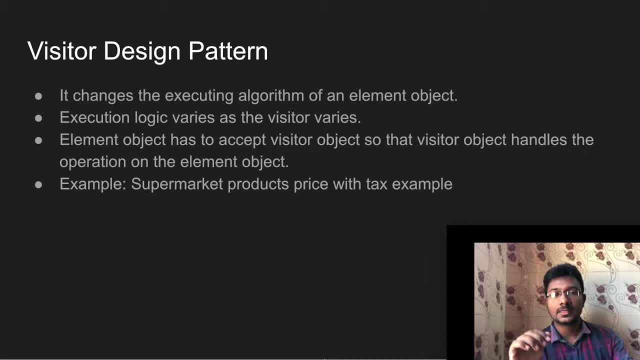 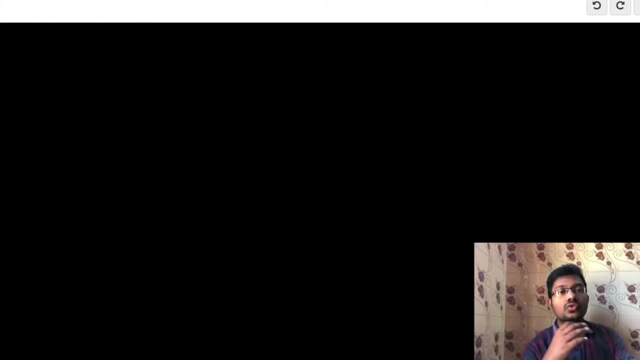 So please stay tuned to this series. Before discussing about the principles, what we can do is we will try to explain this visitor design pattern using some real-life examples. So further, I am taking a shopping mall example. So this is a shopping mall. Let 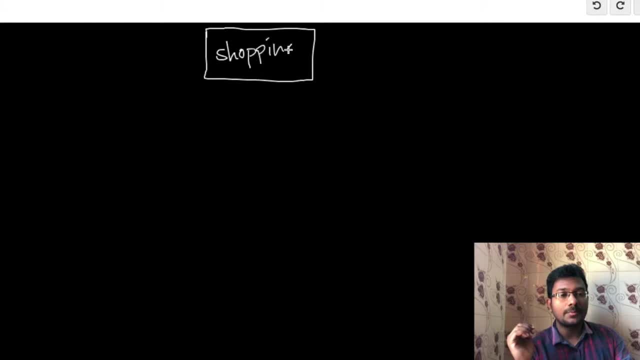 us consider: this is a shopping mall. So in shopping mall we can buy many kinds of products. For example, we can buy food products, we can buy toys, we can buy dress, we can buy utensils. So these are the four categories of products that we can buy. 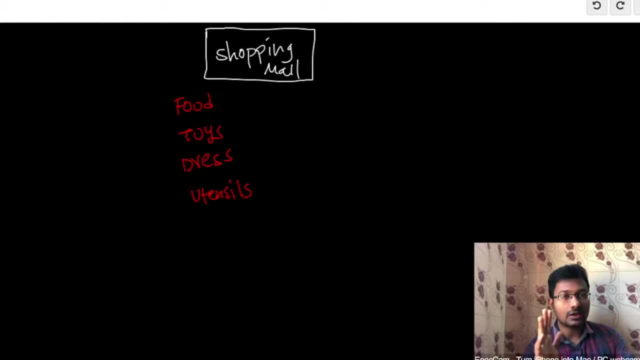 can buy in shopping mall. So let us consider a scenario where a country changes the tax percentage for each category or every month. So let us consider three months: Jan, Feb and March. So these are three months that we are considering. So that country changes the 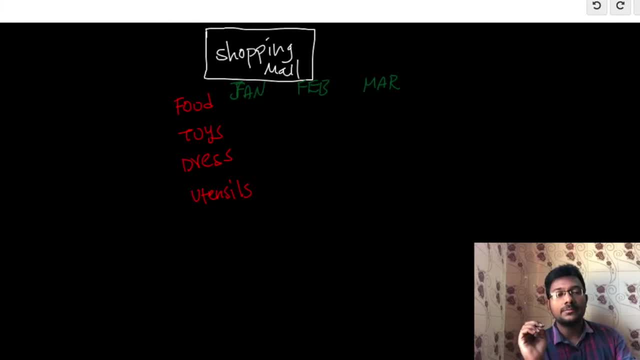 tax percentage on each month, So for each month. for example, if that country decides 5% tax for food products for Jan month and 10% for toys, and 15% for dress and 10% for utensils For February month, the tax percentage varies. So the government decides that the tax percentage of food is 10%. 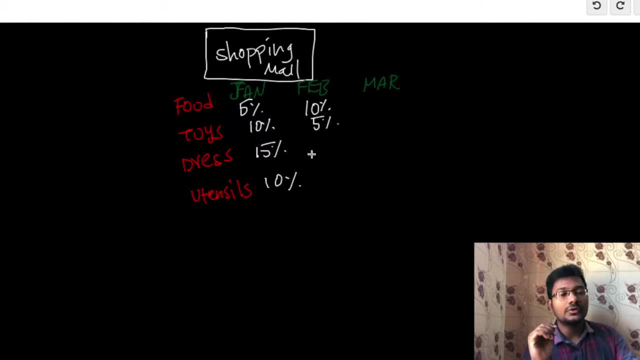 for February month: 5% for toys, 15% for dress and 15% for utensils. For February and March, once again it will be: has 5% loss, 10%, 20% and 30%. So here for each month the tax is getting. 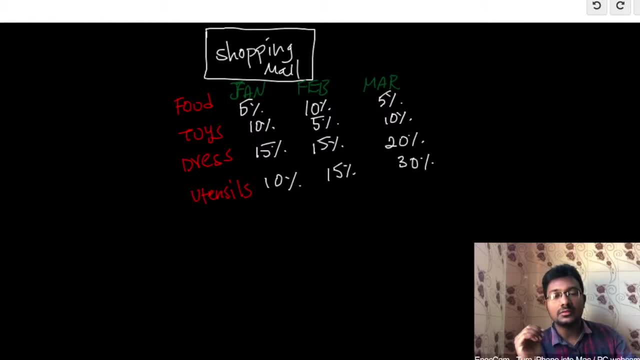 varied. so we can consider that food, toys, dress and utensils are elements. so we can consider elements. so we can consider these things are elements and we can consider 3, 12,, 15, objects: Jan visitor. Feb visitor. March visitor. So here for each month, the tax. 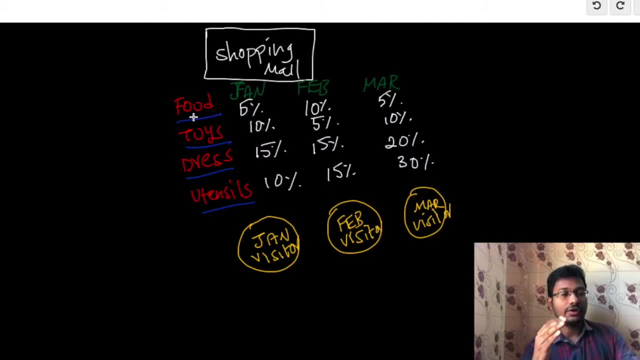 is getting varied, So based on element, for example, food, toys, dress utensils are the elements For food. the tax percentage for Jan month is 55%, so that could be handled by the visitors. So these are the three visitors who are. 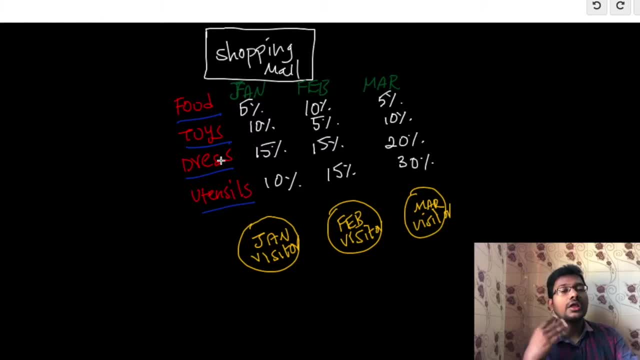 visiting the products or elements and they are determining or executing some algorithm. So if suppose, if Jan visitor receives the food, toys, dress utensils or elements, then it determines the tax percentage for that month and then the next visitor comes for the next month, which means February. 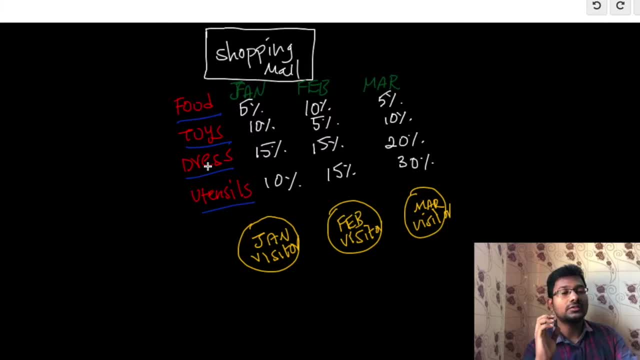 the February visitor is visiting food, toys, dress and utensils and it is determining the tax percentage. and then March visitor is visiting the elements- food, toys, dress and utensils- and then it is determining the tax percentage for that month. So here this visitor is playing a major role. This visitor is 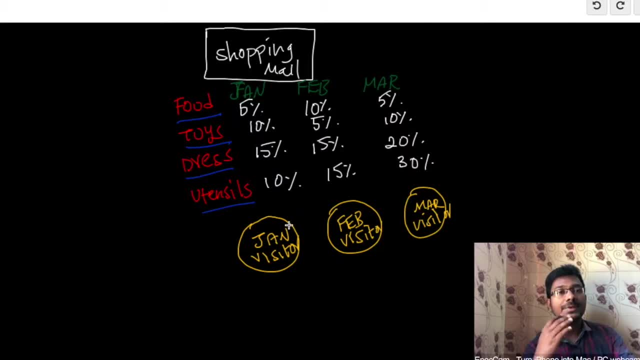 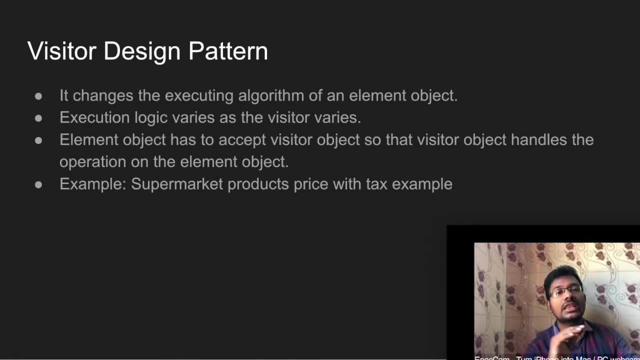 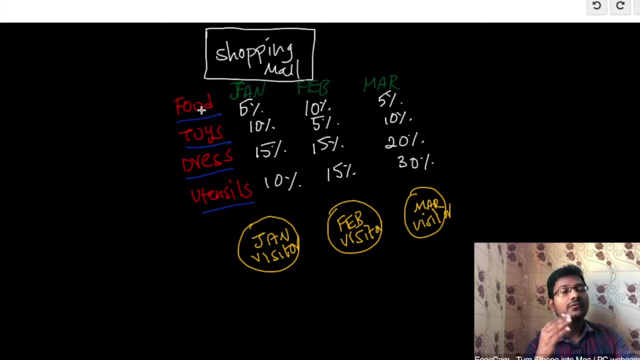 determining the tax percentage for the elements based on various criteria. So that's these points. It changes the execution algorithm of an element object. So these are the elements: food, toys, dress, utensils. The execution algorithm varies as the visitor varies, So execution logic. 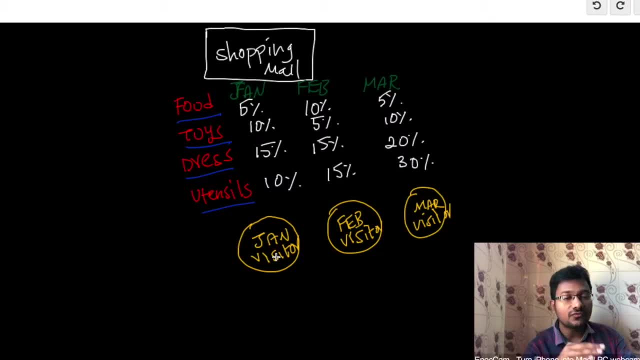 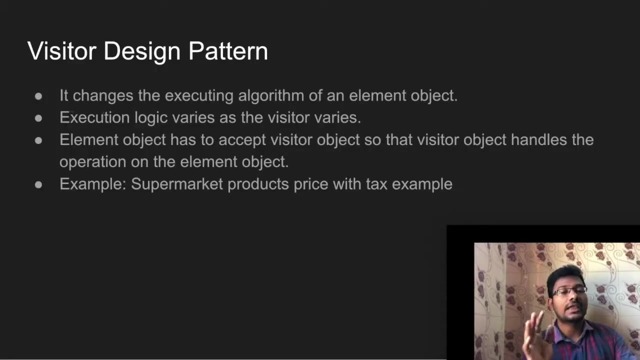 varies as the visitor varies Here. if Jan visitor visits food products, then it determines the tax as 5%. If February visitor visits the food product, then it determines the tax percentage as 10%. That's the second point explanation and the third point states that element object has to. 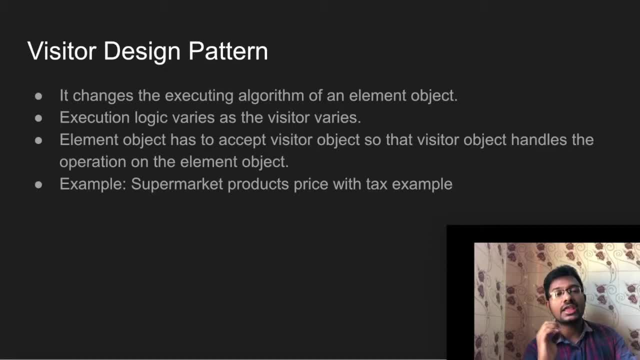 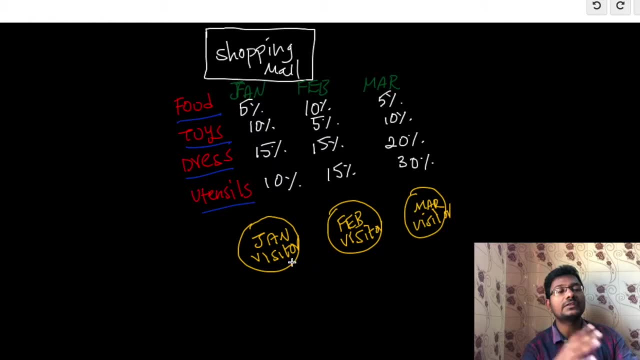 accept the visitor object so that the visitor object handles the operation of the element object. These are the four elements. These four elements need to accept the visitor object so that the visitor object can execute its algorithm on the elements. So this is the simplest example where the 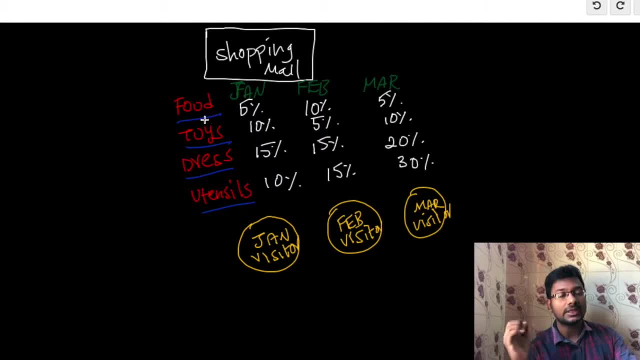 visitor dis체가 pattern is accomplish and then tree is shown in the title of the behavior in the kanjiว as well, as시 is playing a major role in real life exam in real time. so we can consider another scenario where visitor design pattern is playing a major role in our real life. for example, if suppose we are: